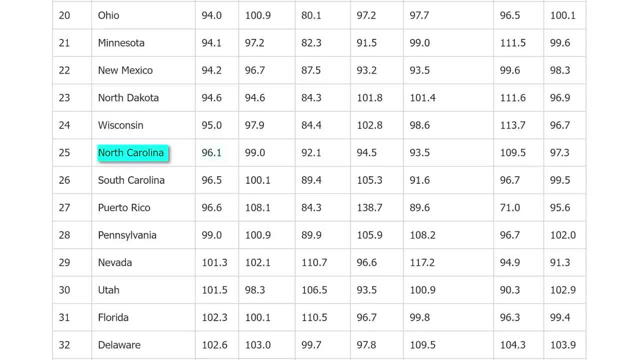 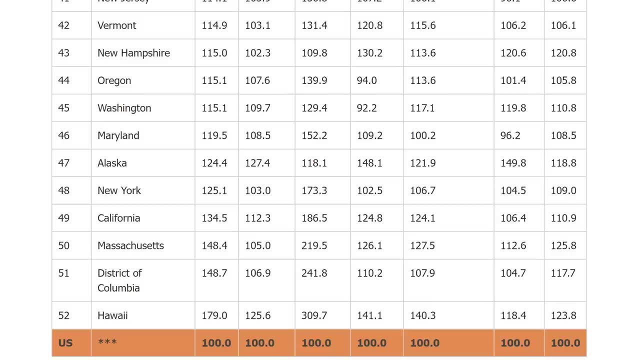 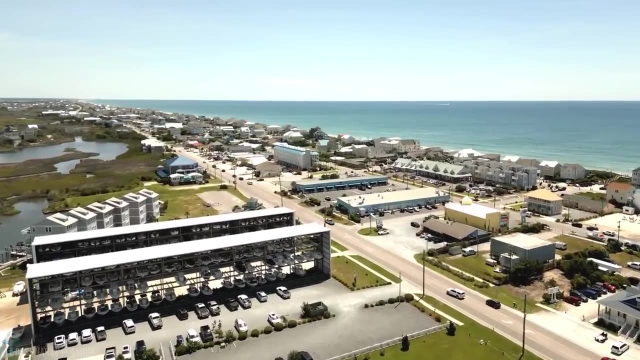 North Carolina has one of the lower costs of living in the US, with an index of 96.1.. For reference, the most expensive state in the country is Hawaii, which has a cost of living index of 179.. The reason for this has to do with housing, as North Carolina has some of the more affordable. housing in the US Number two strong economy. For those concerned about inflation and a rising cost of living, they may be more likely to move to a place with a strong economy, and North Carolina fits that description. For starters, its economy is fairly diverse. The state has industries ranging from 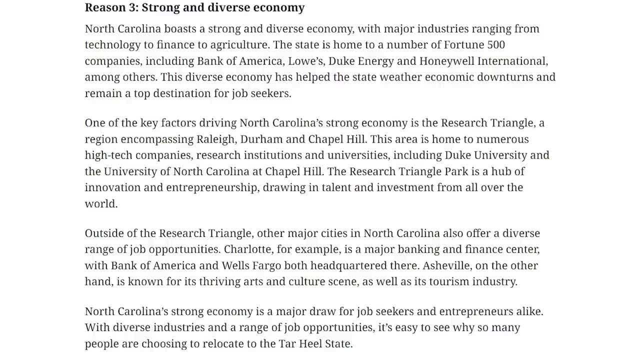 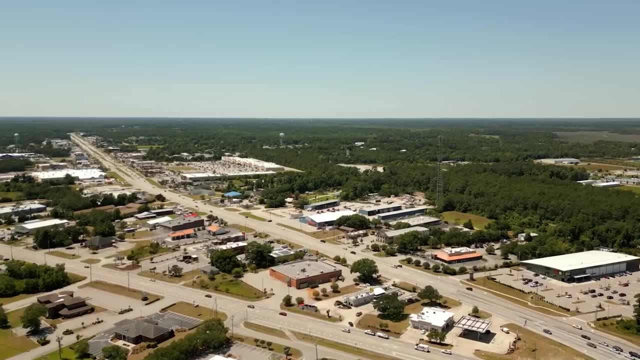 agriculture to finance to tech, and major forestry to agriculture. The state has a lot of companies, including Fortune 500. companies like Bank of America, Lowe's and Honeywell International are positioned there. As a result, its diverse economy means that it's more resilient when things 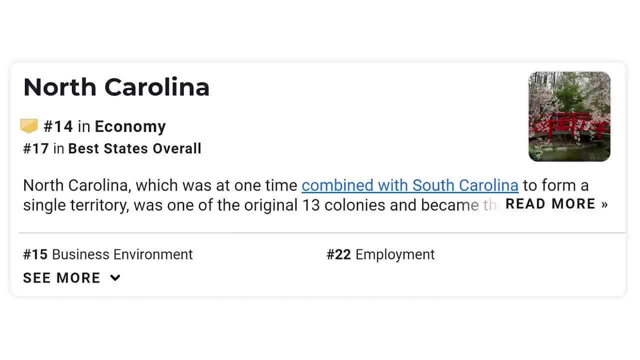 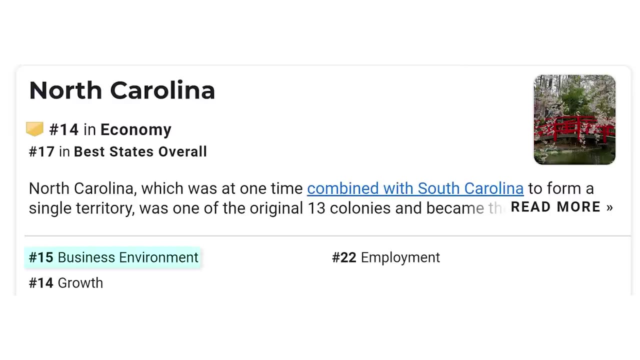 get tough elsewhere. This may be one of the reasons that US News and World Report ranked it the 14th best state in terms of the strength of its economy, according to factors like its business environment, labor market and economic growth. Specifically, it ranked 15th in terms of: its business environment- 22 for employment and 14 for growth. And North Carolina's growth was pretty impressive, seeing a 1.2% job growth. For reference, the state with one of the lowest-ranked economies, Louisiana, reported a 0.1% job growth. 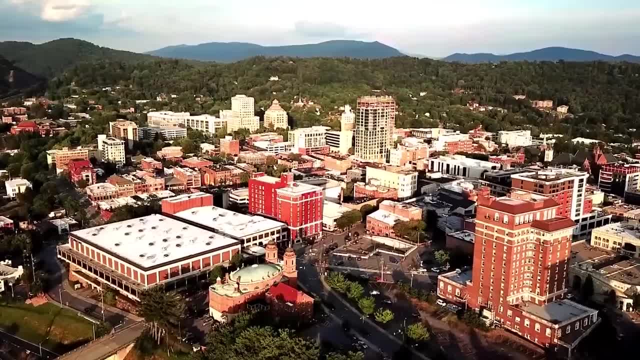 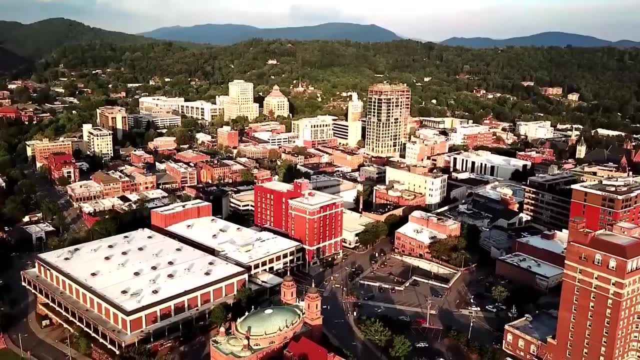 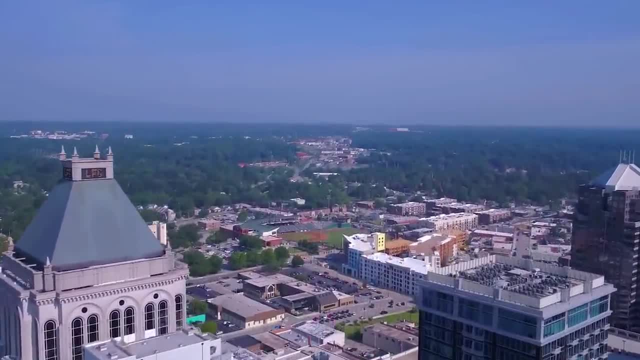 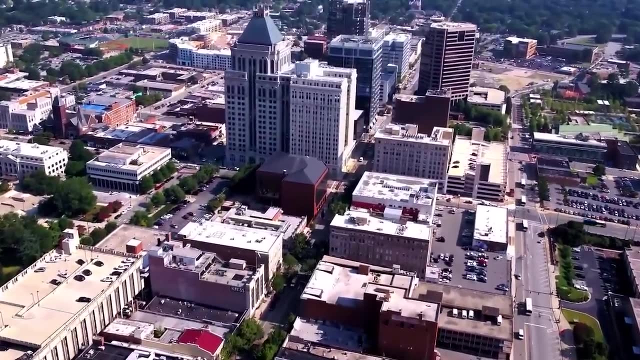 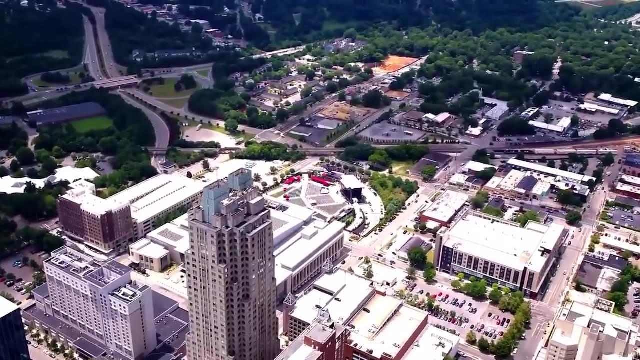 has launched a robust advertising campaign in recent years that's aimed at recruiting people and businesses to the state. Maybe you've even witnessed some of these ads yourself while listening to a podcast or watching a video online. This campaign launched back in 2021 under 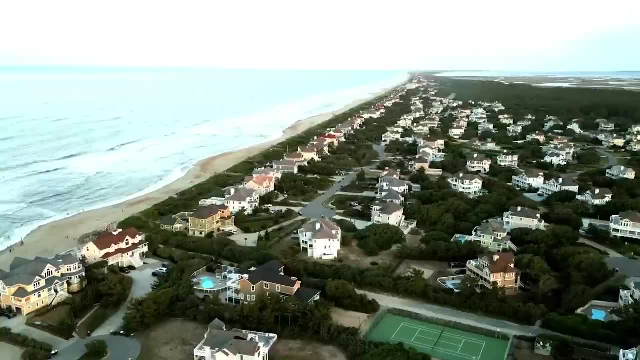 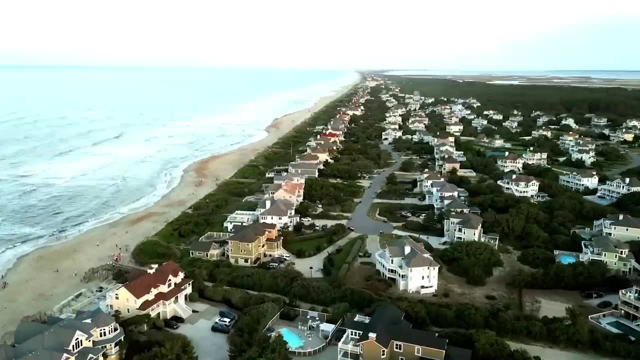 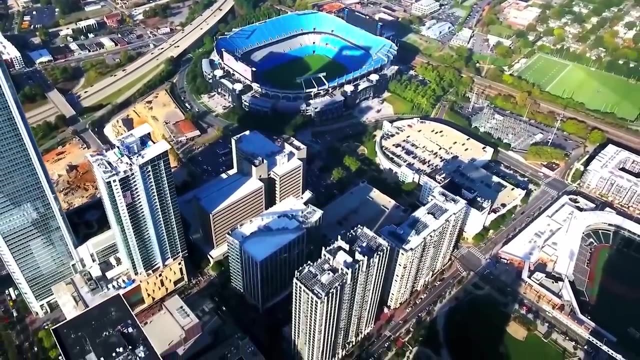 the Economic Development Partnership of North Carolina. It was started in response to the pandemic, with the campaign being an attempt to bring jobs and tax dollars to the state as a part of North Carolina's pandemic recovery plan. And the campaign isn't small. All in the state has 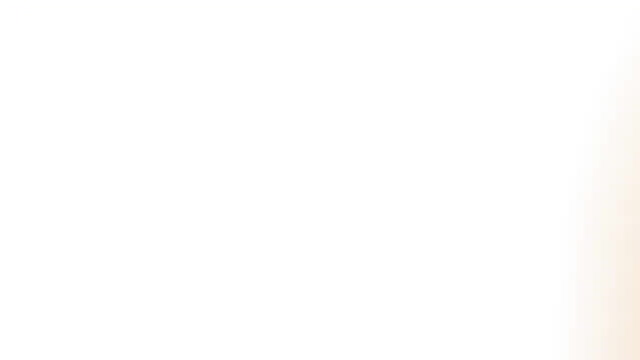 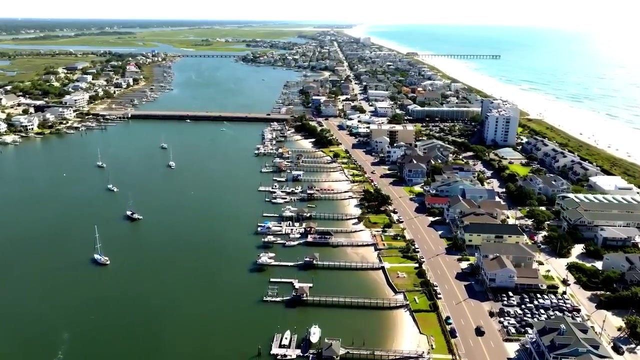 spent $2 million on advertising. Number four: cost of housing. Another factor that may be pulling people to North Carolina and contributing to its significant population growth is the affordable cost of living. According to a report by the New York Times, the state has spent $2 million on. affordable housing for the state. The median sale of a home across all of North Carolina was a little over $370,000 as of May 2023. Compare that to the national median sale, which was $418,000 in the same time period, and it's pretty clear how much more affordable North Carolina real estate can be. 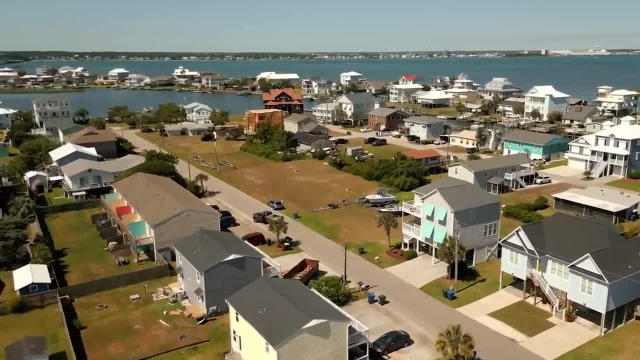 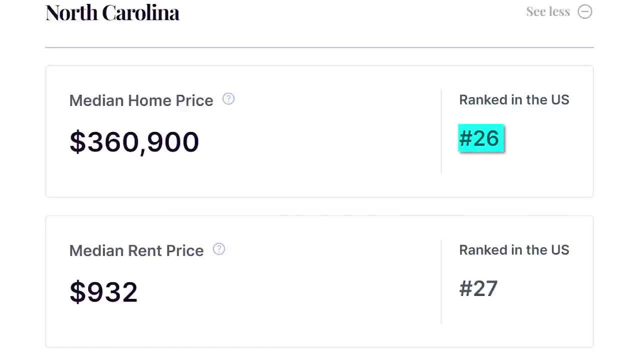 But it's not just May that saw better numbers for North Carolina. This has been a consistent theme for the state. For instance, the state has spent $2 million on affordable housing for the United States. Wise voter ranked North Carolina number 26 in terms of the best states to buy a. 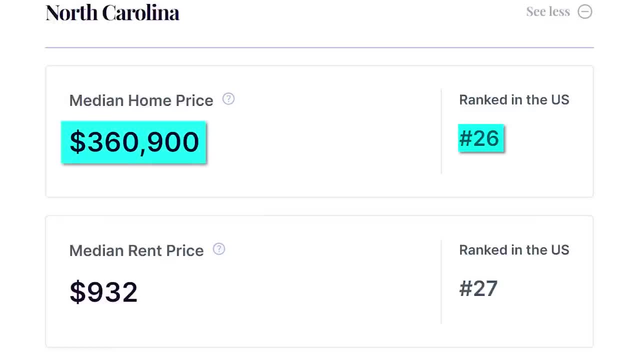 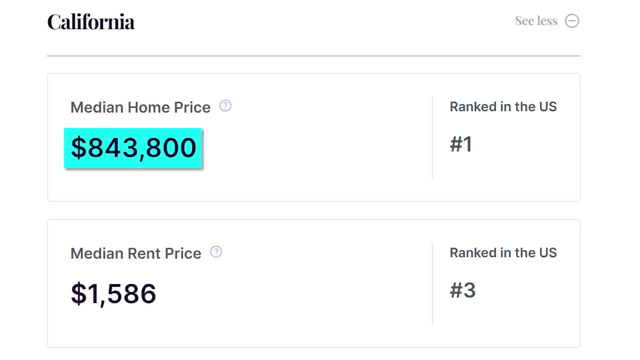 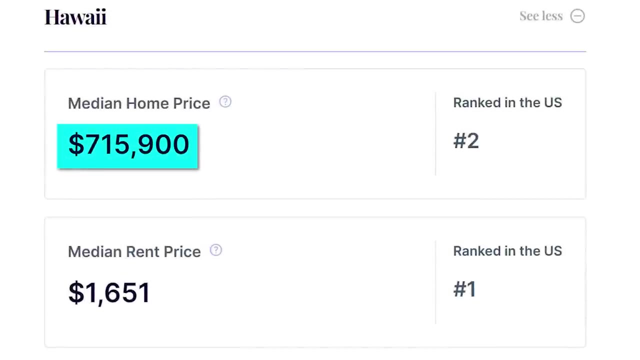 home, citing its median home price of about $360,000. The most expensive states for reference are California, with a median home price of over $843,000,, and Hawaii, with a median home price of about $716,000.. The good news continues for those who rent. North Carolina ranked number 17 in terms 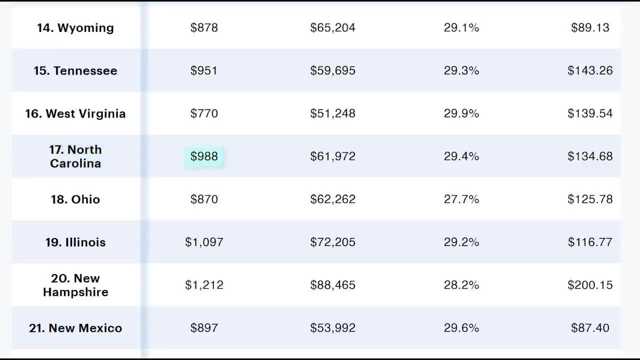 of best states to rent in, with a median rent for a one-bedroom of $988 and an average of 29.4% of income going to rent. That's below the national average of $1,085 for a one-bedroom and well. 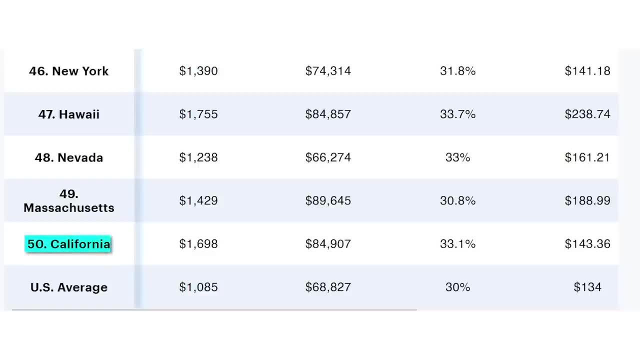 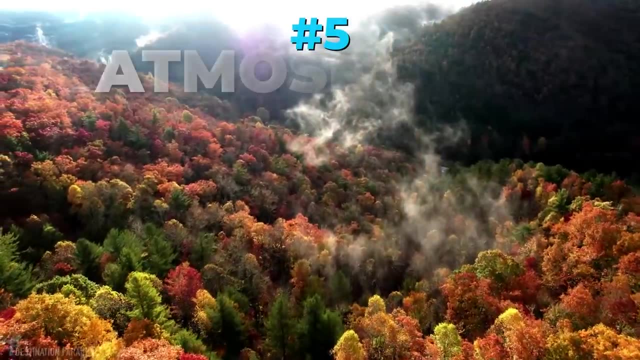 below the most expensive state to rent in California, where the median rent for a one-bedroom is $1,698.. Number 5. Atmosphere. According to OneReport, North Carolina is the most expensive state to rent in in the United States. 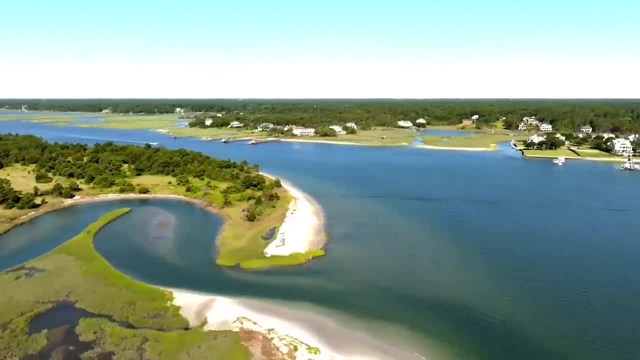 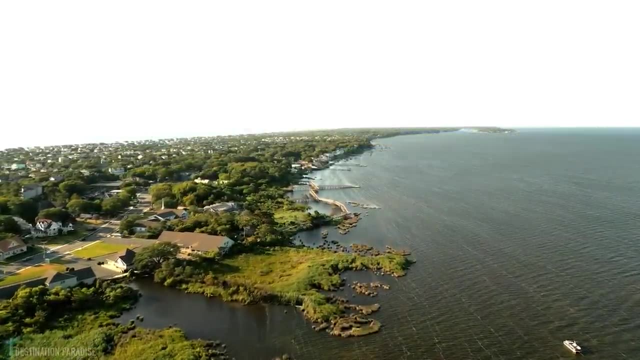 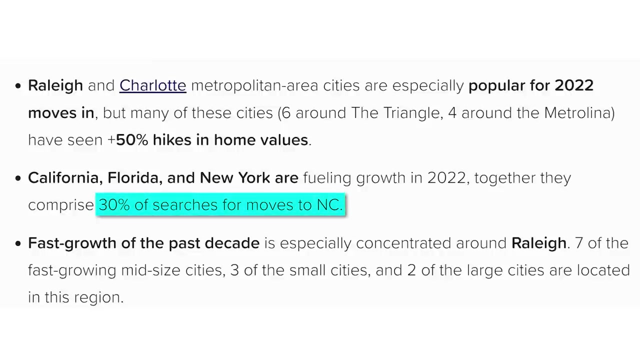 People are increasingly looking to move to areas with lots of open space, and North Carolina offers that, especially for those moving from more dense states. Recently, 30% of all those who searched online about moving to North Carolina were from California, Florida and New York, states that are 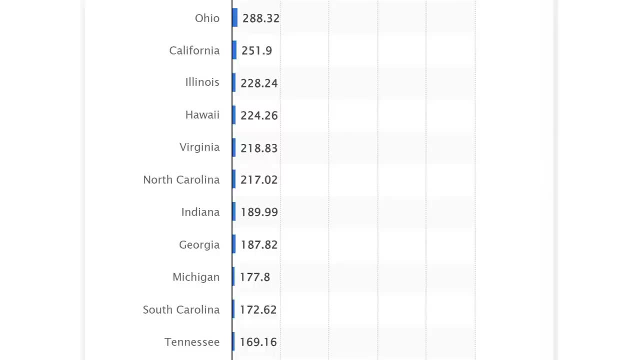 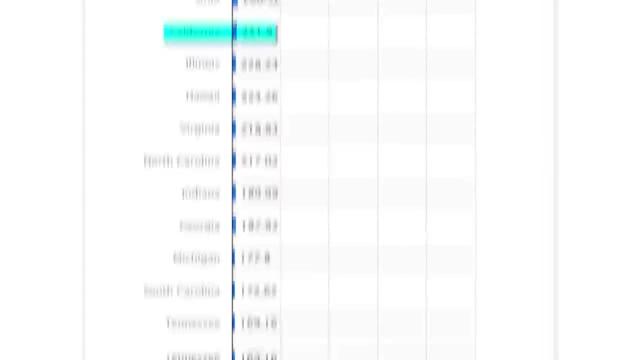 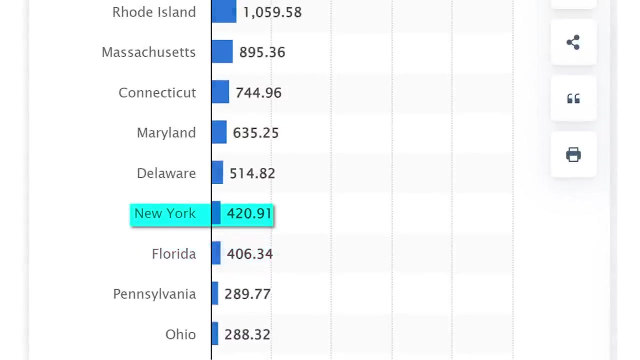 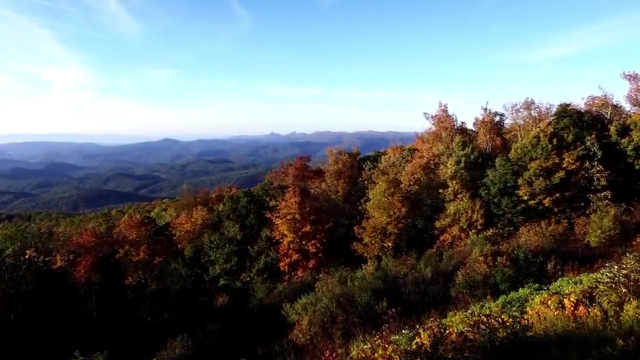 California is 251 people per square mile, Florida is 406, and New York is 420,- almost double North Carolina's. Another reason people are moving to North Carolina is for the weather, as people are seeking out states with more mild temperatures. Averages across the state range: 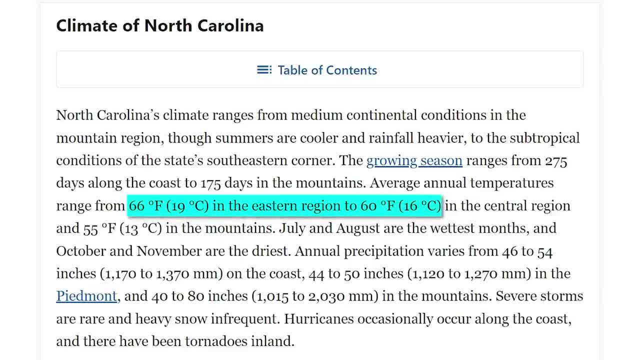 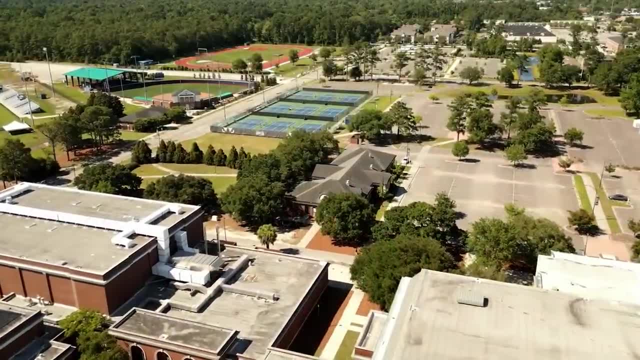 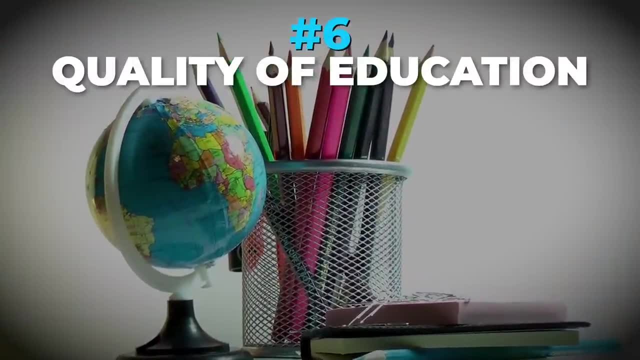 from 60 to 66, depending on where you are, and residents here enjoy mild winters and balmy summers, me summers. Essentially, you get four seasons without the extreme temperature swings that some other states have. Number six: quality of education For those with children moving. 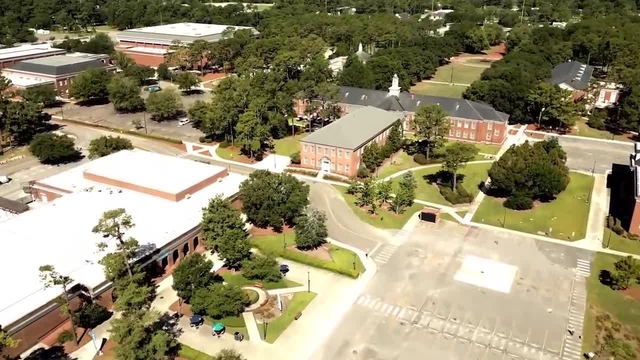 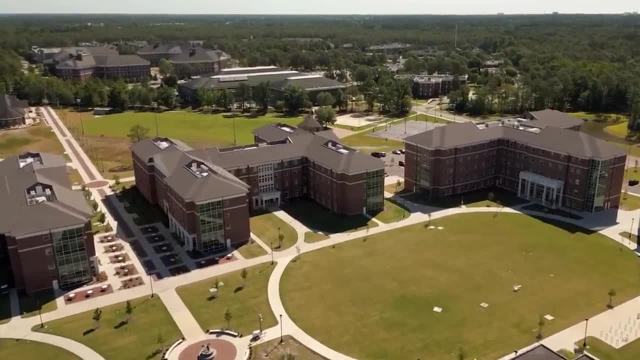 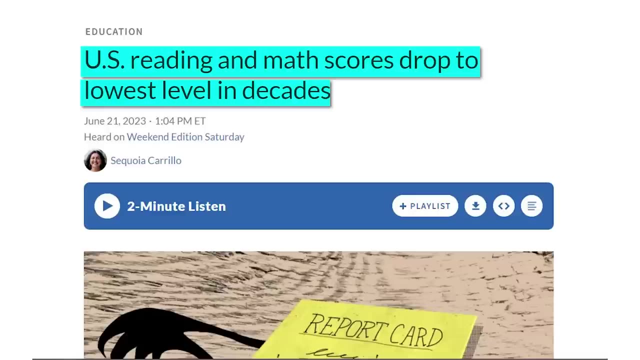 somewhere with good quality. public schools has become more important now than ever. That's because the quality of public schools nationwide has been declining. For instance, a new report showed that math and reading scores recently plummeted to the worst levels in decades. Those moving to North Carolina may not have to worry about these issues, though, and that might be. 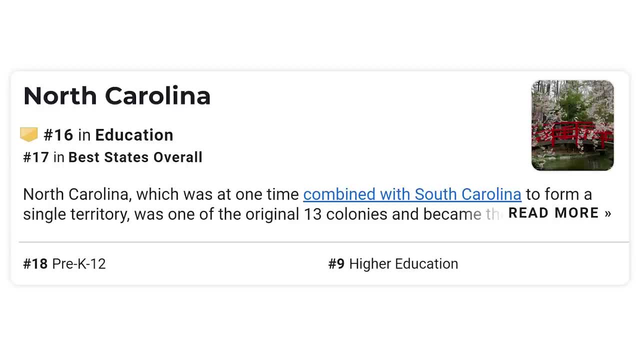 another draw for those who are moving there. According to US News and World Report, North Carolina is number 16 in the country in terms of both its higher education and quality of public schools, grades kindergarten through 12th grade. The state's average high school graduation for 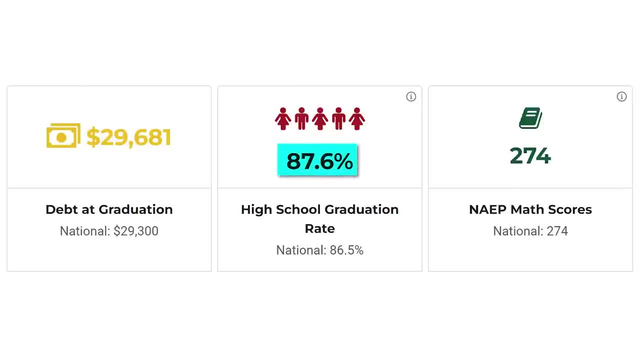 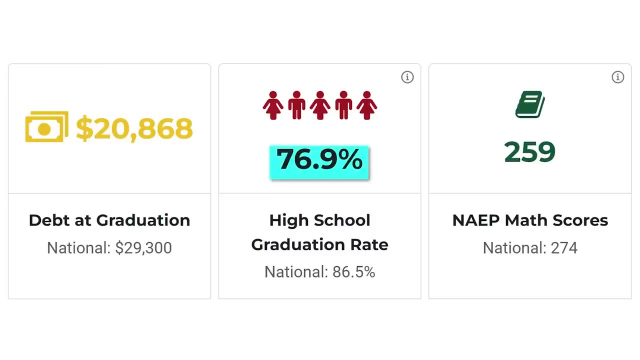 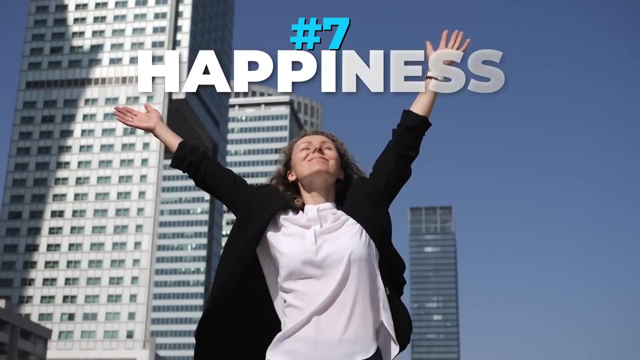 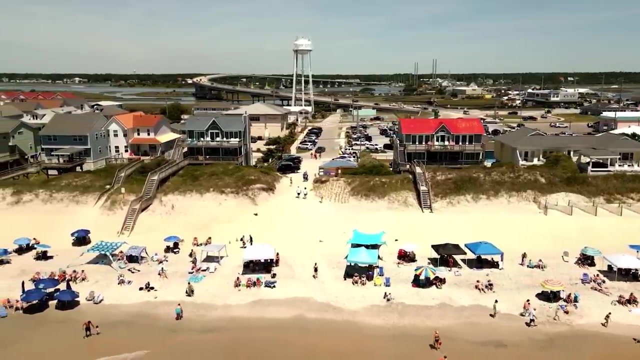 instance, is 86%. For reference, the state with the lowest education ranking, New Mexico, has an average high school graduation rate of 76.9%, over 10% lower than North Carolina's Number seven, happiness. I'll preface this by saying that happiness rankings are likely not the main reason people are moving. 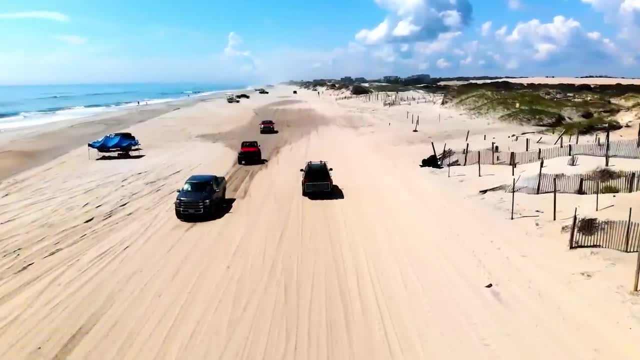 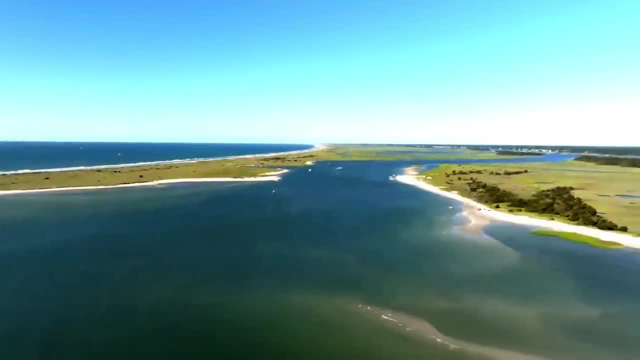 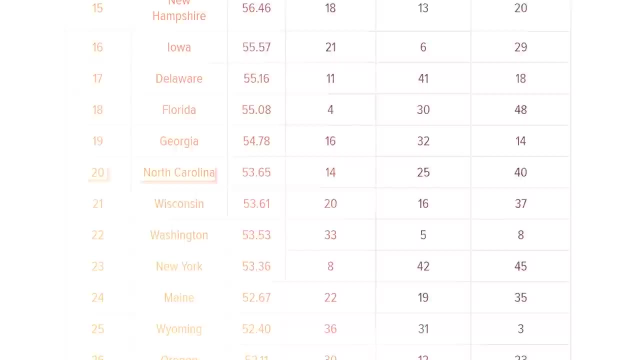 here. However, if you visit a place and people seem genuinely happy, it may be an additional factor. And North Carolina, according to a study by WalletHub, is one of the happier states in the country, recently ranked number 20.. To determine the rankings, WalletHub ranked each state. 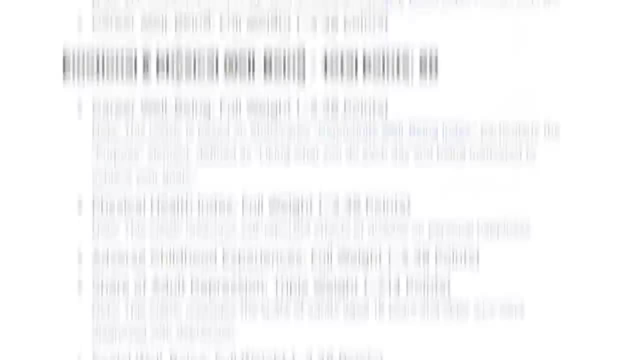 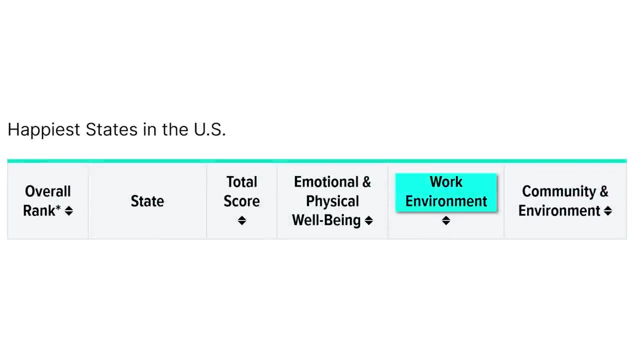 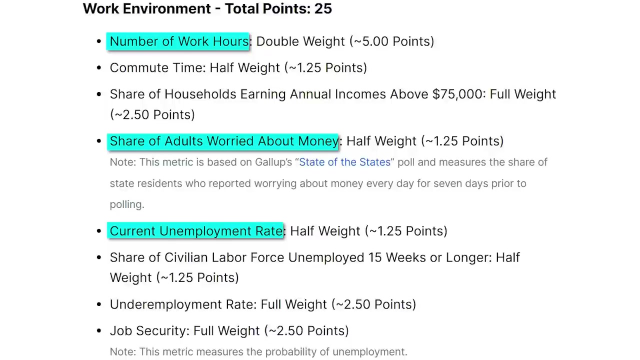 according to factors like emotional and physical well-being, which includes career well-being, physical health and share of adults with depression. Work environment, which includes the average number of work hours, share of adults worrying about money and underemployment rate. And finally, community and environment, which includes metrics like 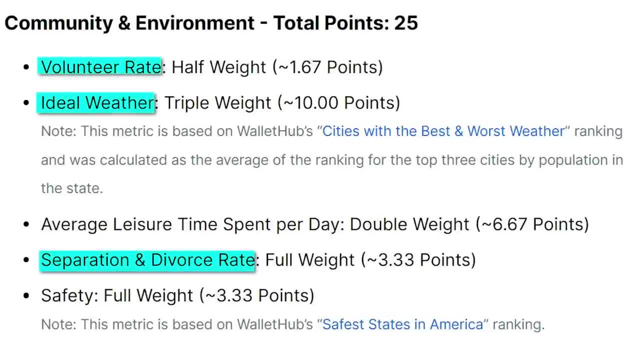 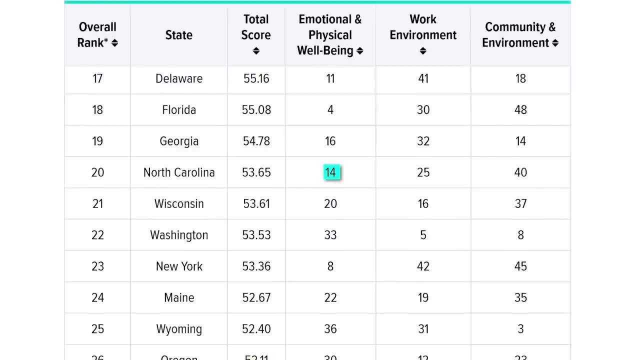 volunteer rate, divorce rate and ideal weather. As I mentioned, North Carolina came out number 20 overall and, notably, ranked number 14 when it comes to emotional and physical well-being. I should note that it ranked towards the bottom when it comes to community and environment. 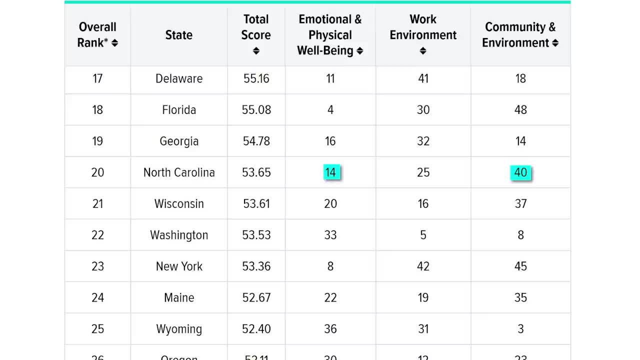 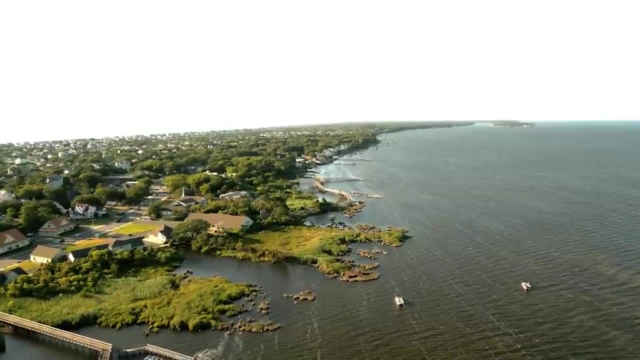 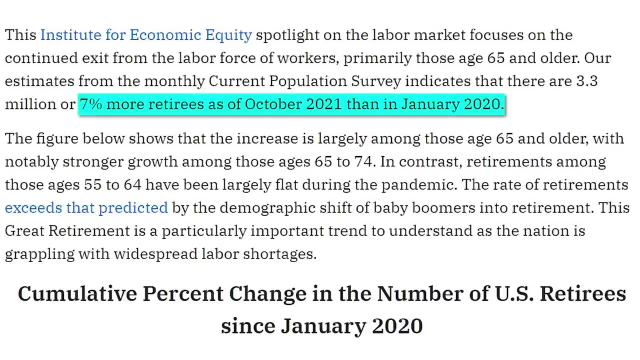 However, this wasn't enough to offset its high scores in other states. 8. Retirement Opportunities: The number of retirees has seen an increase in recent years. In October 2021,, for instance, the number of retirees was 7% higher than the number in January of 2020,. 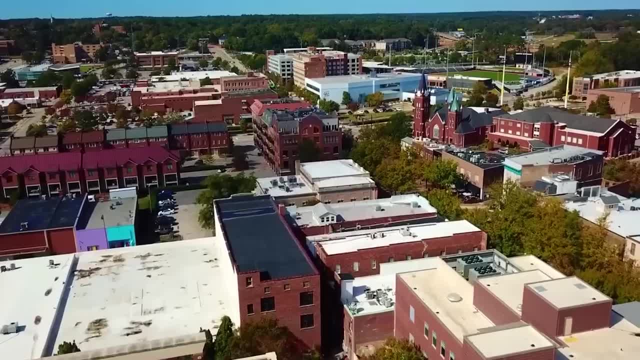 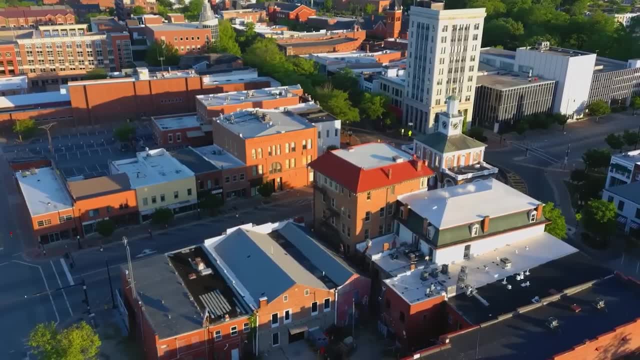 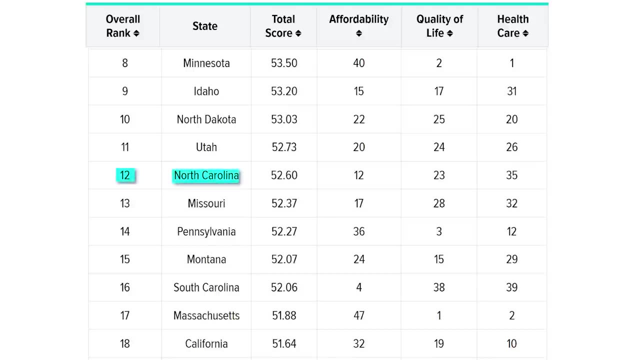 equating to about 3.3 million people, And with the cost of living on the rise and climate change impacting some retirees' planning, North Carolina has increasingly been seen as a top retiree. Recently, it was ranked as the 12th best state to retire in according to metrics including: 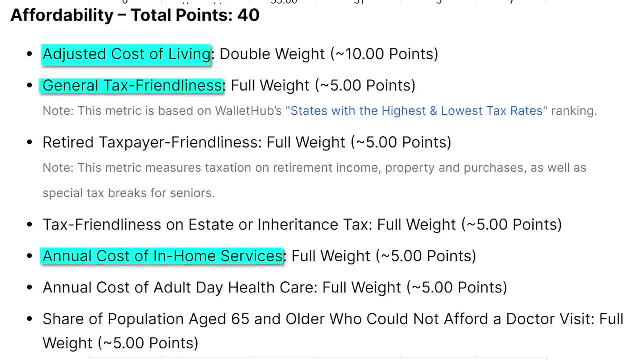 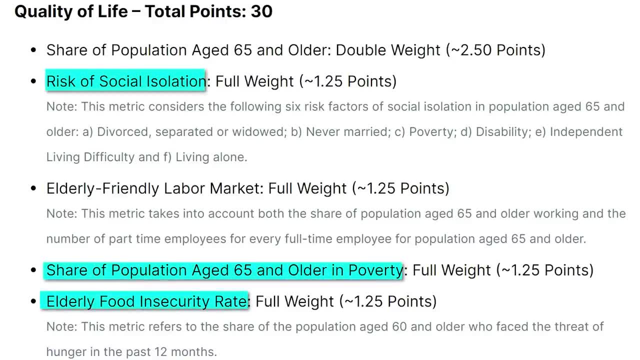 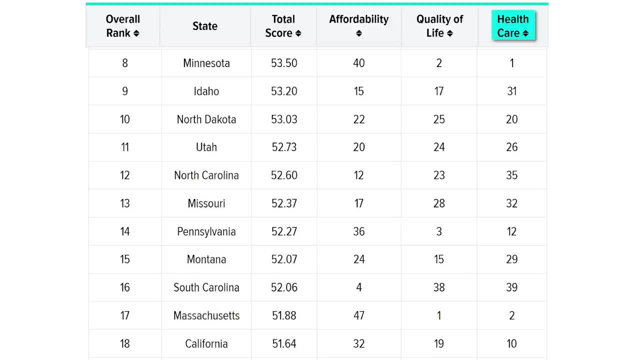 affordability, which includes cost of living, tax-friendliness and in-home service costs. quality of life, including social isolation, elderly food insecurity, rate and share of the population ages 65 and above living in poverty. and health care, including physicians per capita. 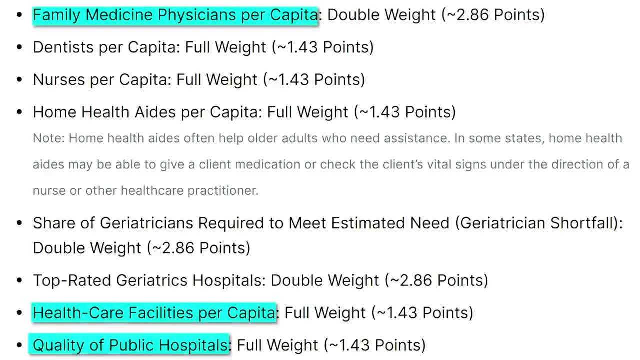 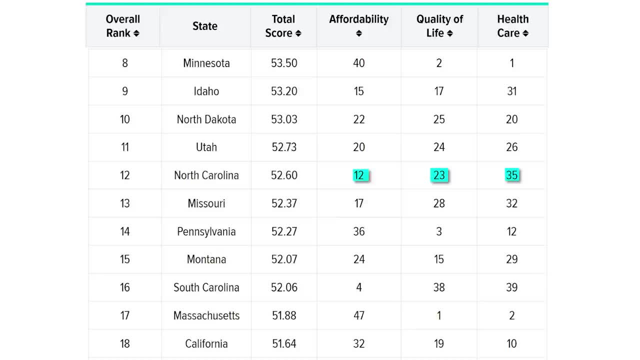 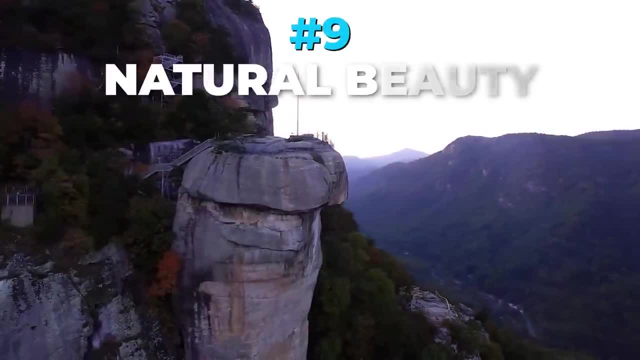 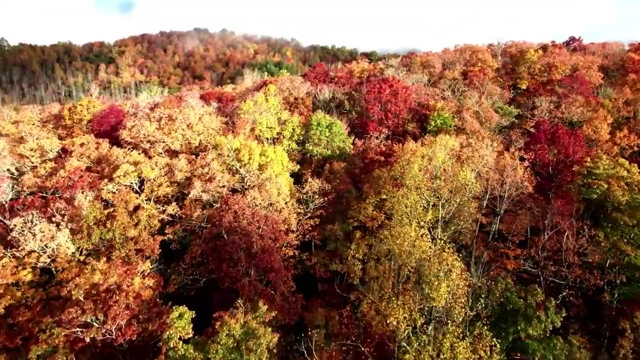 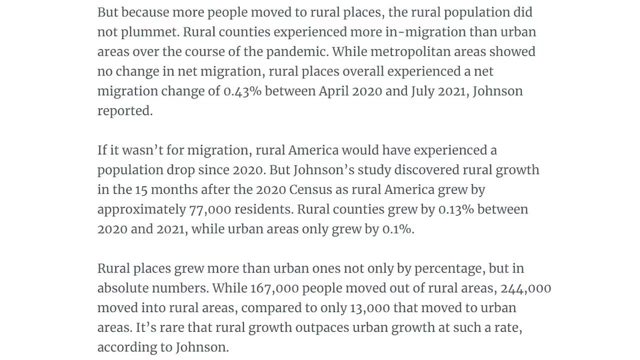 health care facilities per capita and quality of life. 9. Natural Beauty: In a movement called the Rural Migration Trend, Americans are increasingly moving to rural areas, showing their wish to be closer to nature. Between 2020 and 2021,, 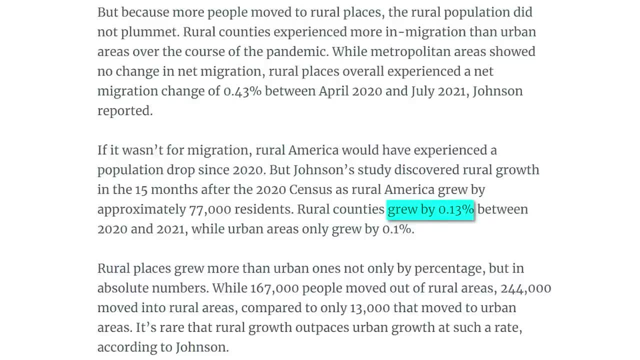 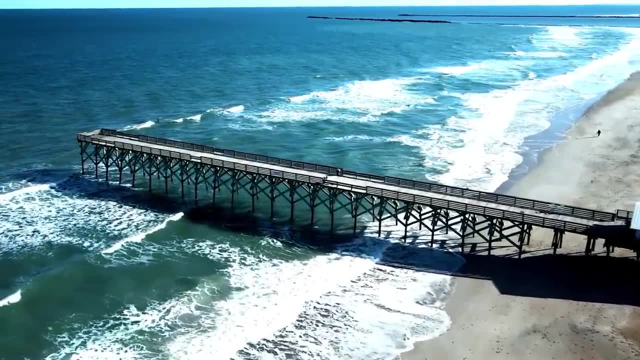 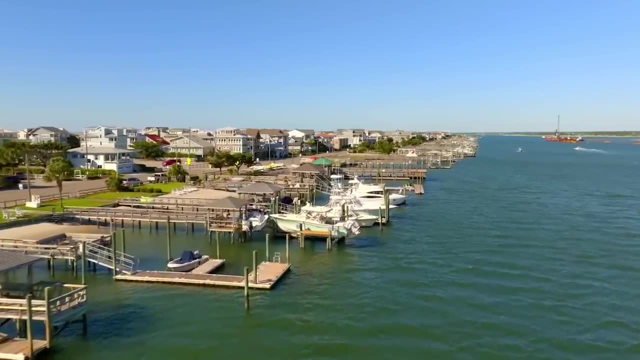 rural areas grew by 0.13%, compared to a 0.1% increase in urban areas. This might not seem like a huge difference on the surface, but it is. when you consider this in the context of migration changes over time, As in the past, urban areas have historically seen more growth than rural. 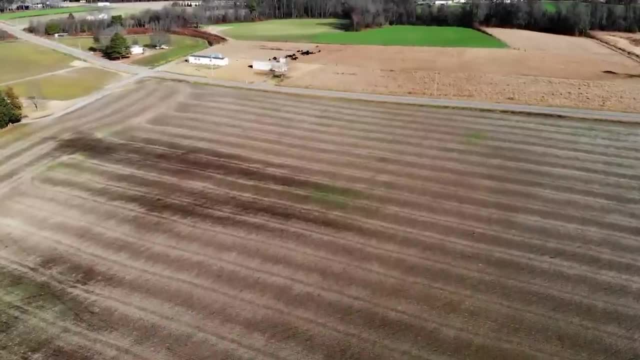 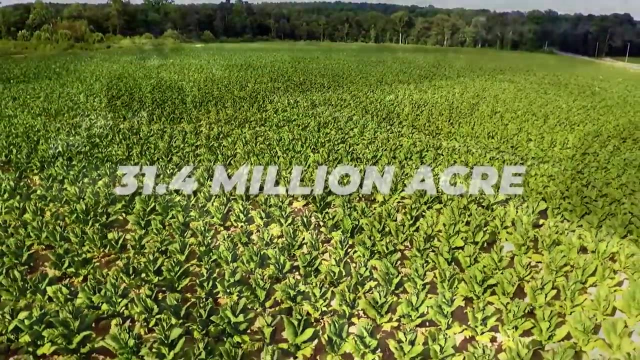 ones. While North Carolina isn't completely rural, it has plenty of nature to enjoy Out of North Carolina's third-largest rural area. North Carolina is the third-largest rural area in the country, With 31.4 million acres. for example, 5 million, or about 16% of these, are public lands. 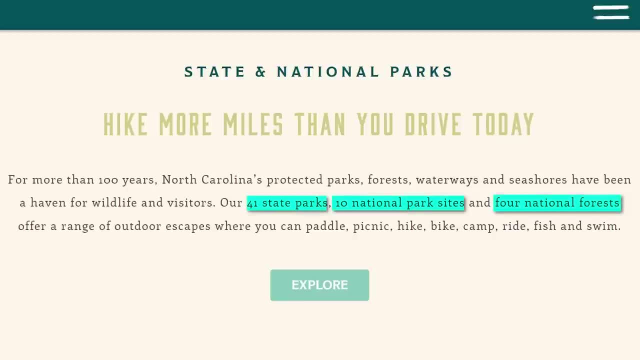 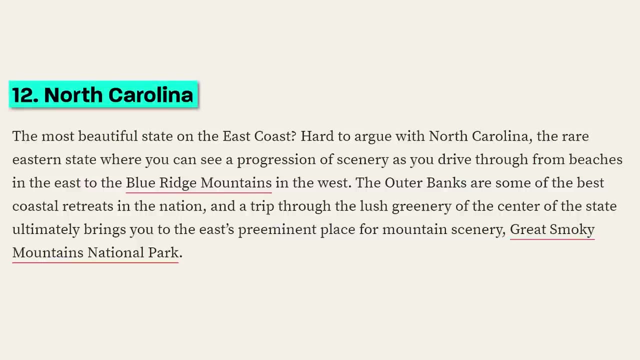 For instance, North Carolina has 41 state parks, 10 national park sites and 4 national forests, and Thrillist ranked it the 12th most beautiful state in the country, citing its beaches, Blue Ridge Mountains and incredible Great Smoky Mountains National Park.